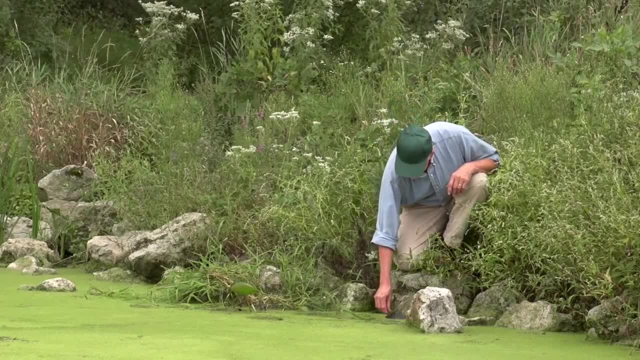 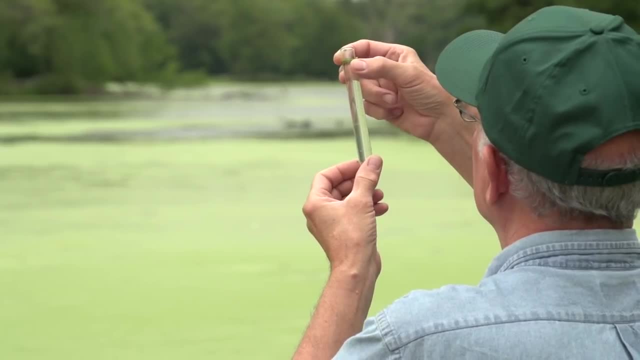 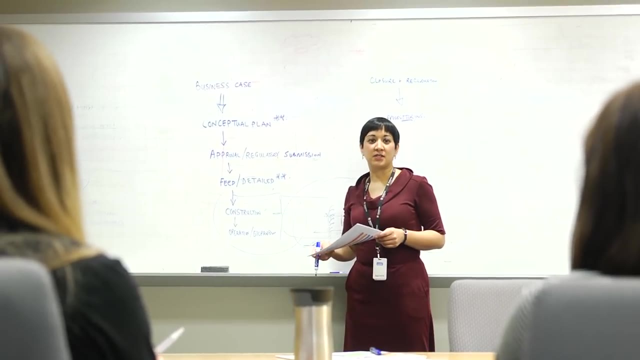 of the environmental aspects of a site. We might do an assessment of soil and groundwater to determine if there's any contamination on the site and then develop a remediation action plan and execute the remediation. We could do environmental audits of industrial sites. We might advise clients or government agencies on how to manage the environmental impact. 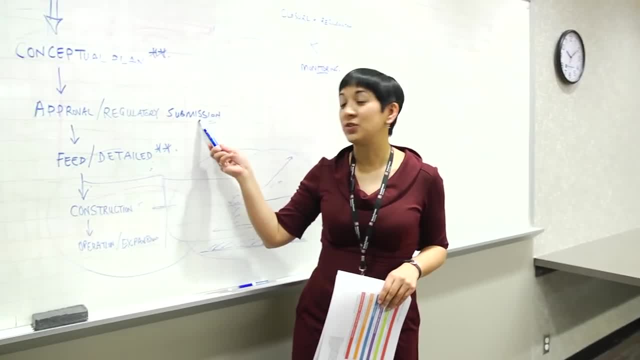 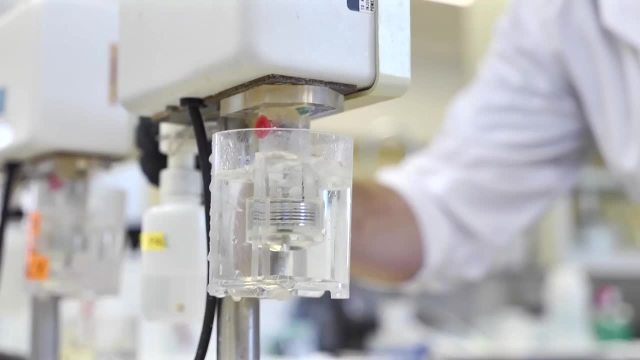 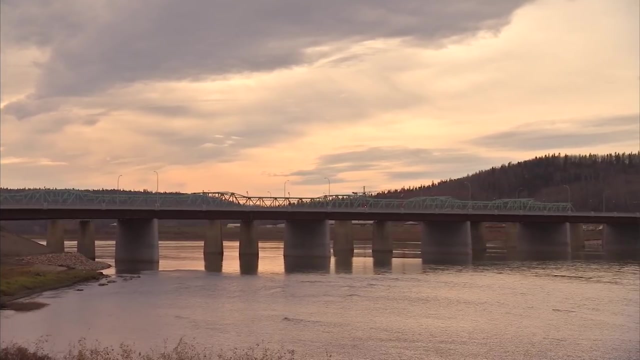 on the site. We might do environmental audits of industrial sites. We might advise clients or government on policies or how to implement policies and environmental regulation. We also might be involved with water quality assessments, both for potable or industrial waste. We can also be involved with large infrastructure projects such as bridges, roads, also determining 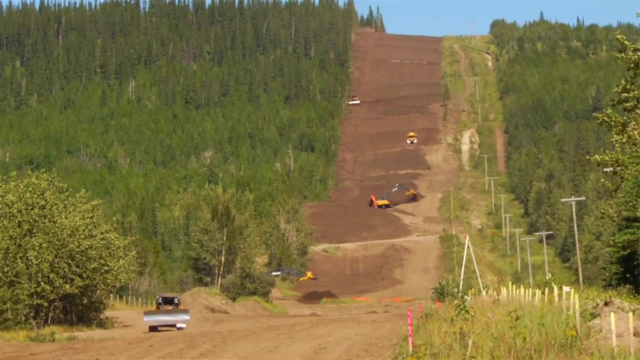 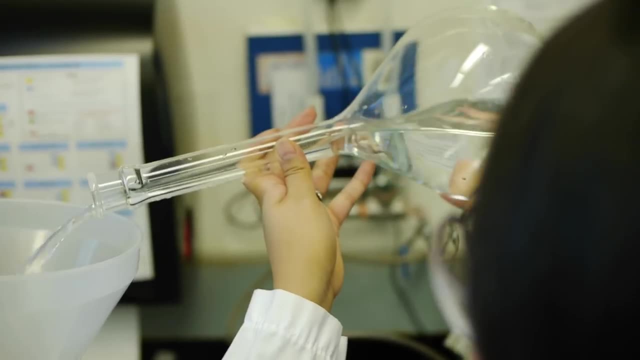 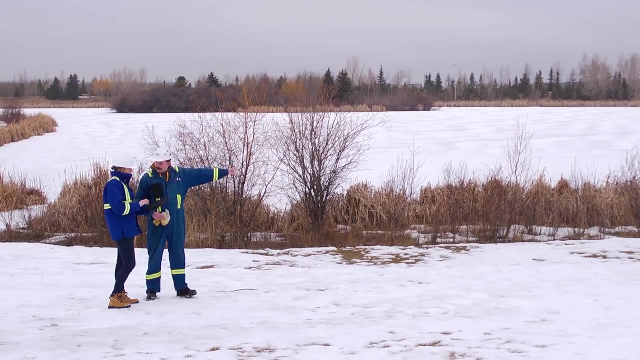 what the environmental impact would be from that development. This profession is multidisciplinary. We often are working with scientists, geoscientists, We may be working with lawyers- if there's a legal implication- government agencies and, of course, our clients. So on a day to day, you have to have personal skills. 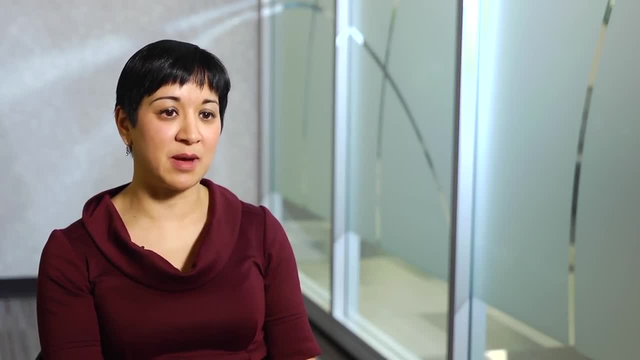 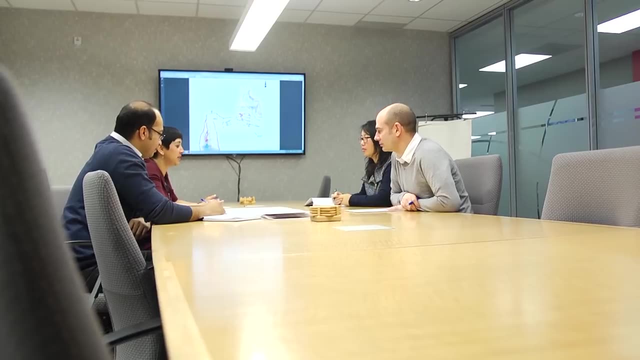 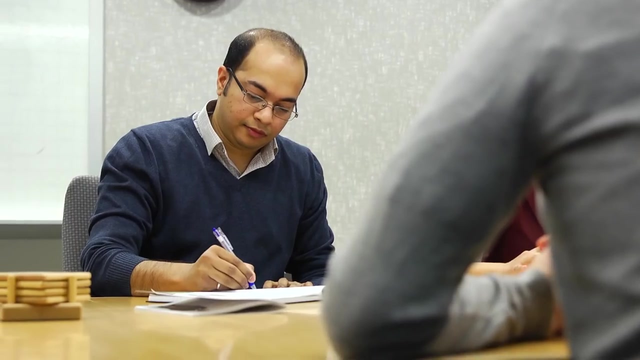 When hiring environmental engineers, we first and foremost look at personality. What we also look for is whether or not they have perhaps a mechanical aptitude. You should be able to think on your feet and independently and be able to seek assistance when necessary. Some environmental engineers work at games. We're going to be working with them on the. 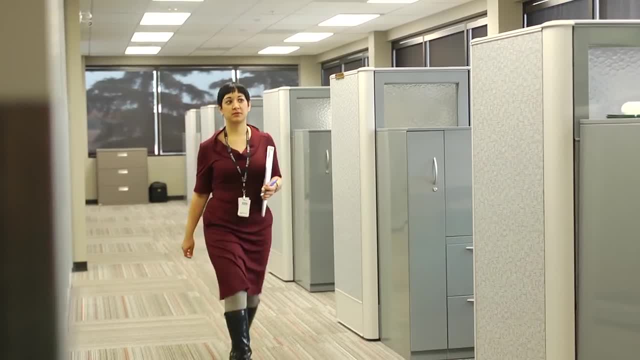 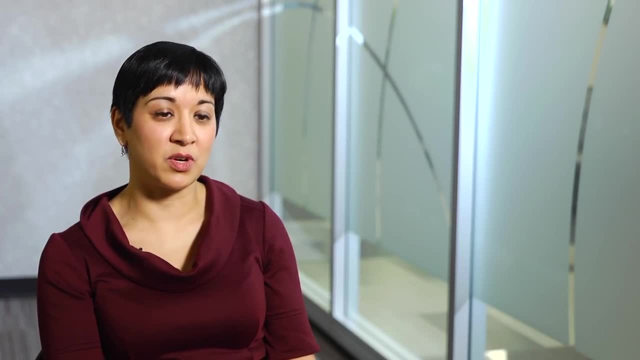 site. Some environmental engineers work at gas plants or remote locations, or they might be working at a head office. The job can definitely lead to travel. I've had the opportunity to work abroad. Last fall I was actually in Bolivia inspecting different mines to determine the 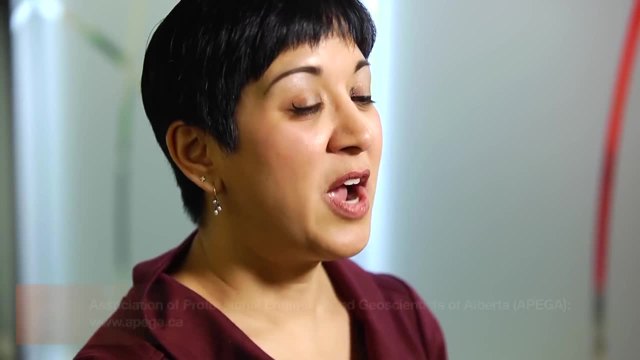 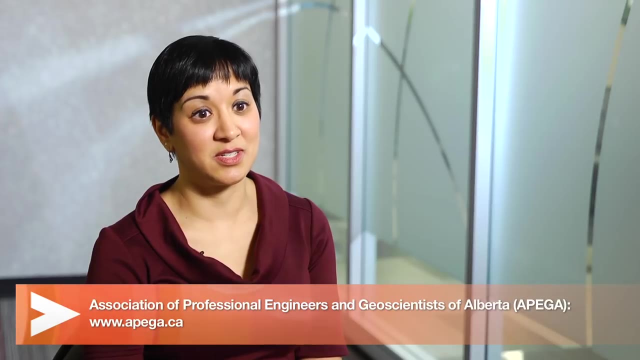 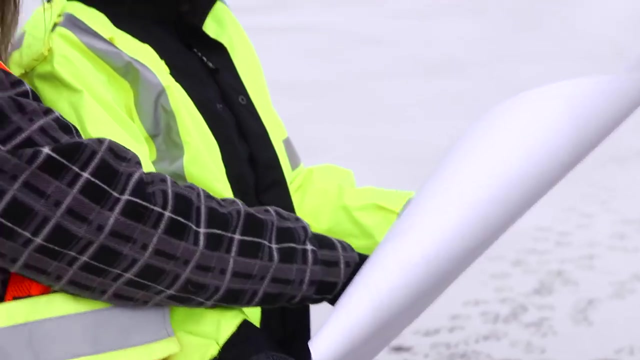 cost of closure and reclamation. To practice as an environmental engineer in Alberta, you have to be registered with the Association of Professional Engineers and Geoscientists of Alberta, also known as APAE. To be a registered professional engineer, you need to have a four-year engineering degree. 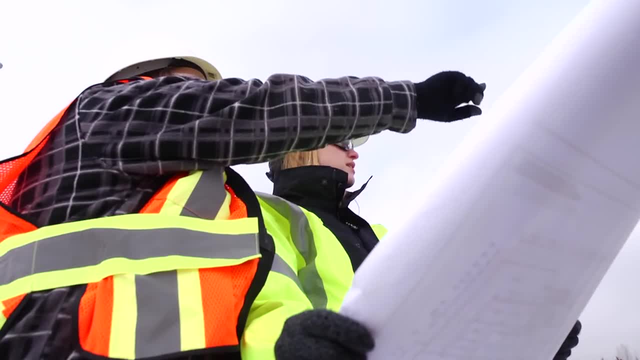 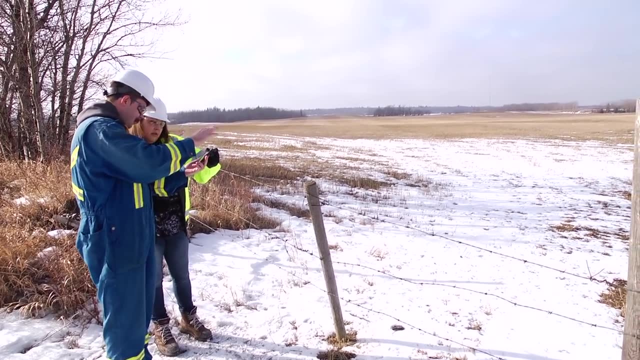 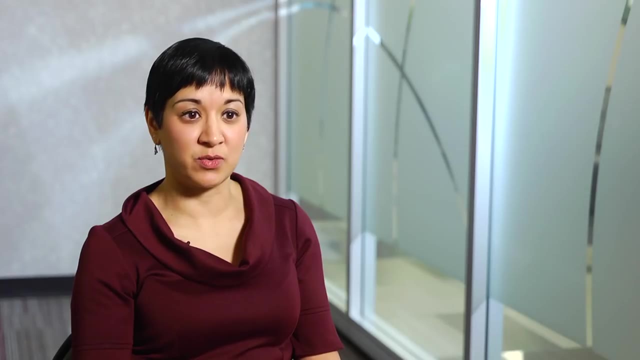 from a recognized institution. You then need to have four years of work experience where you're working under a professional engineer who is in good standing. This career can definitely can lead to advancement anywhere from consulting or higher management positions within organizations or teaching in a university. In my spare time, I like to travel. I like